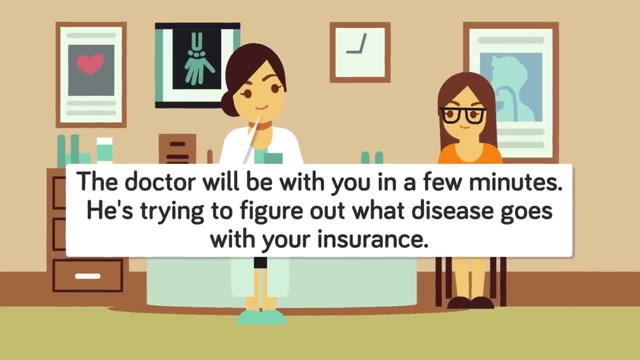 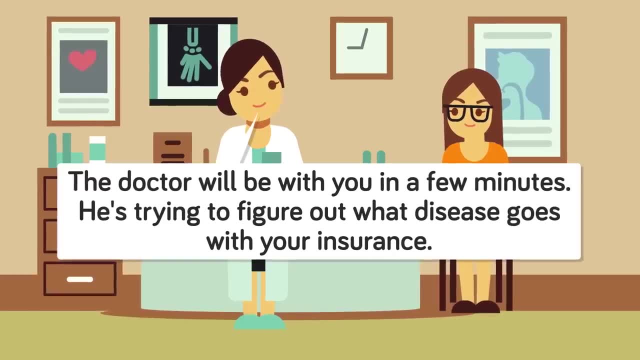 this topic, It came to the conclusion that one must save in America, as sickness or accidents can lead to astronomical bills. The advice it gives: Save for a rainy day in a hospital bed and live a life in line with not getting an ailment. and a life in a hospital bed is often unavoidable, such as diabetes. Shouldn't a developed nation have safety nets in place, though? That's a question many Americans ask. How many Danes go bankrupt because they were unfortunate enough to be hit by a bus? 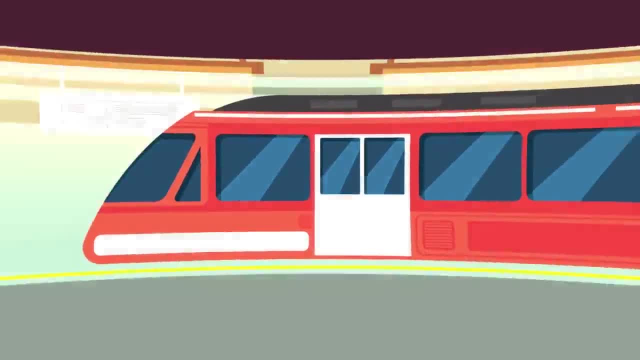 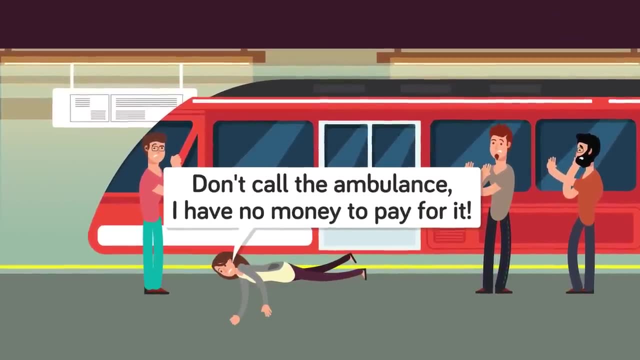 We might recall the recent video that went viral of a woman who had her leg trapped by a subway train in Boston. Don't call an ambulance, she cried, as shocked bystanders witnessed her bone coming through her leg. Why, they asked. She replied: do you know how much an ambulance costs? 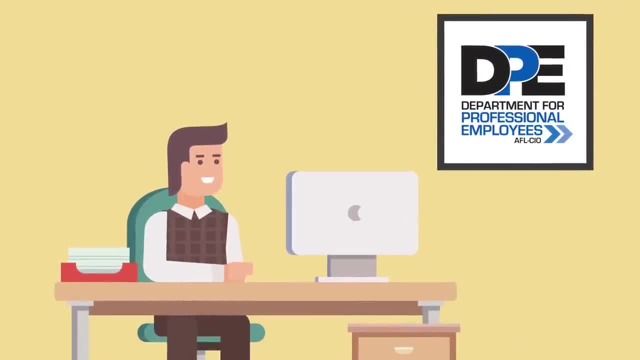 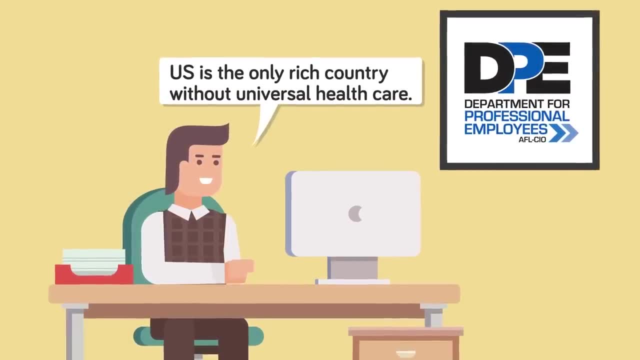 The Department for Professional Employees tells us this: The American healthcare system is unique, at least for an advanced nation. That's mainly because the USA is the only industrialized nation without universal healthcare coverage. That doesn't mean it doesn't spend a lot on healthcare, In fact. 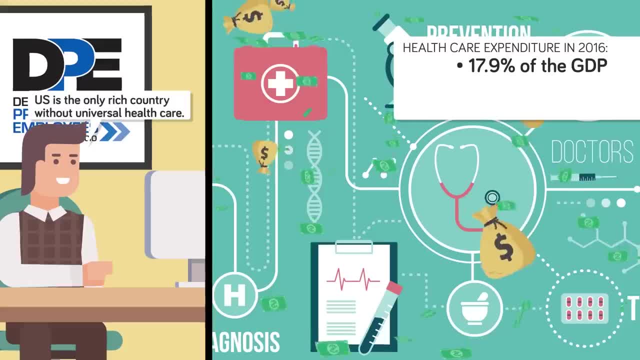 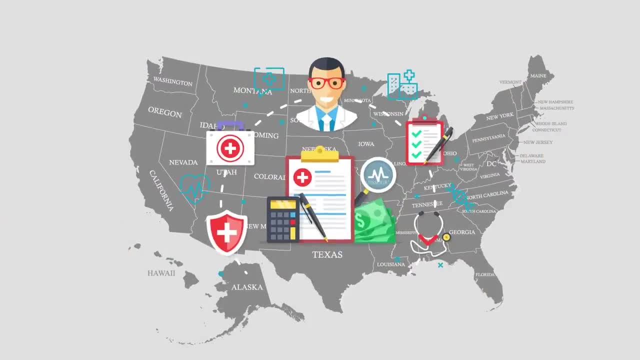 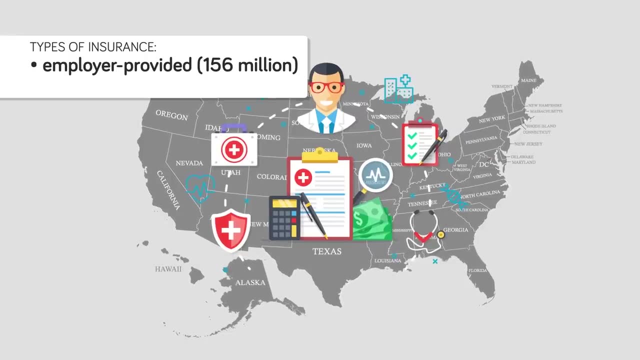 it spends a lot, a hell of a lot: about 17.9% of the GDP in 2016,, or $3.3 trillion. We're told that Americans shop for health insurance just as they shop for anything else, and that's why the system is called a public-private hybrid. 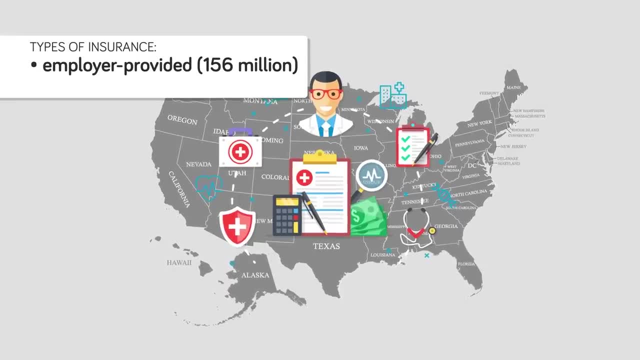 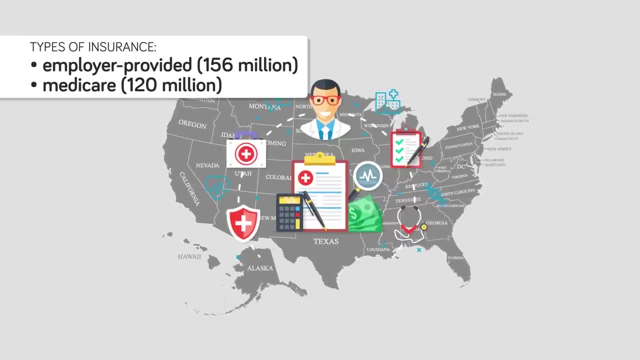 Then you have publicly funded Medicare for old folks and the disabled and Medicaid for the poor. It's thought around 120 million Americans are part of these schemes. That's why the system has been called a public-private hybrid. But when we talk about insurance given or subsidized by employers, 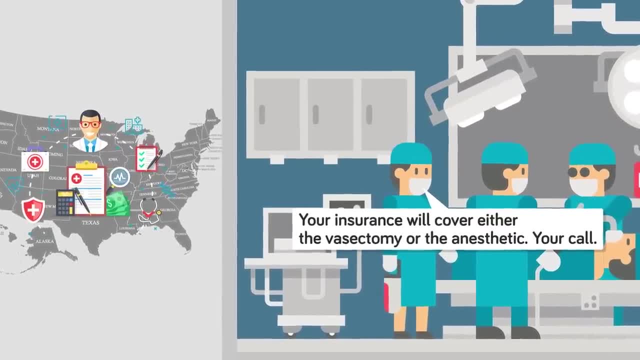 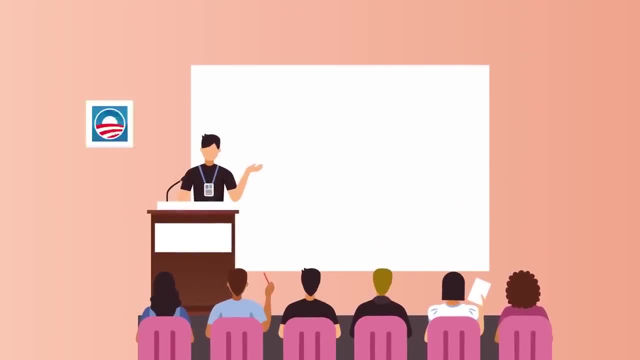 it all depends on what kind of insurance you have. It may not pay for everything, so some people still end up going bankrupt. Then you have the American health insurance system, which is called a public-private hybrid. You have the Affordable Health Care Act or ACA, aka Obamacare, which attempted to make it easier. for employers to give better health insurance plans for their workers. It also made it possible to give the maximum time limit for short-term insurance plans and make it possible for employers to give their workers pre-tax cash to buy their own coverage. As we said, though, 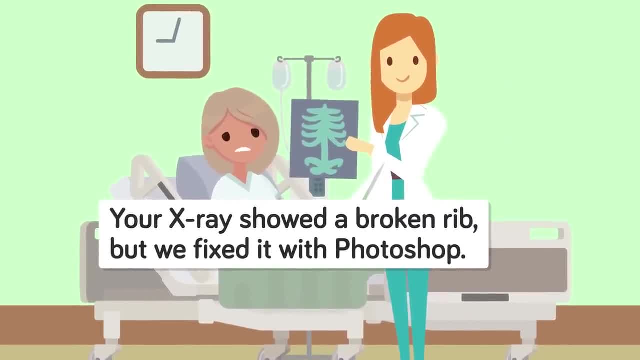 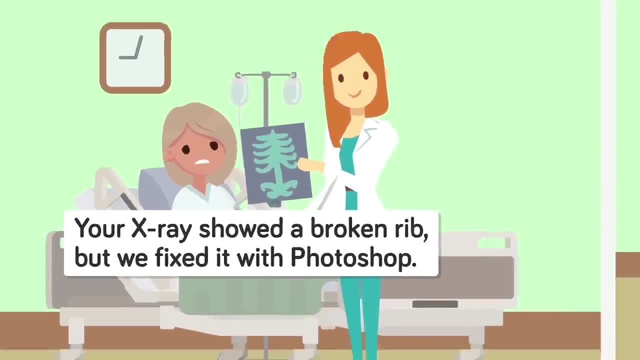 insurance providers don't always give you exactly what you want. They usually have a network of doctors or hospitals and you must use them, and in some cases you are not always covered for the treatment you need. In the past, some people with pre-existing 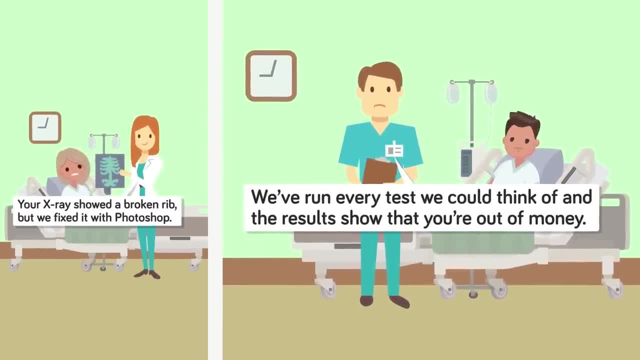 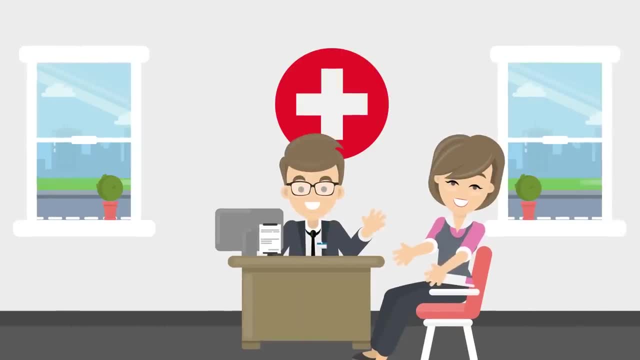 conditions, couldn't afford their insurance or were even denied it, which is just a part of cutthroat capitalism. Obamacare was put in place to prevent this. But let's go back to insurance. When you choose a plan, you must look at these things. 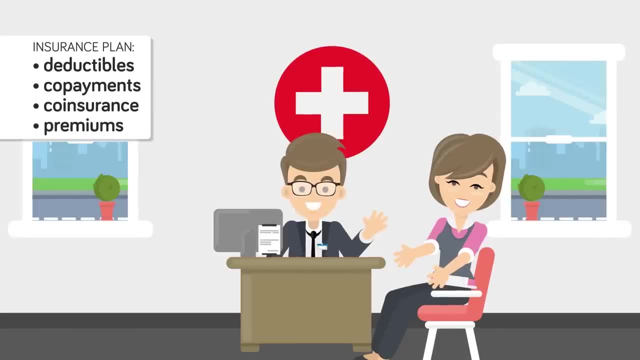 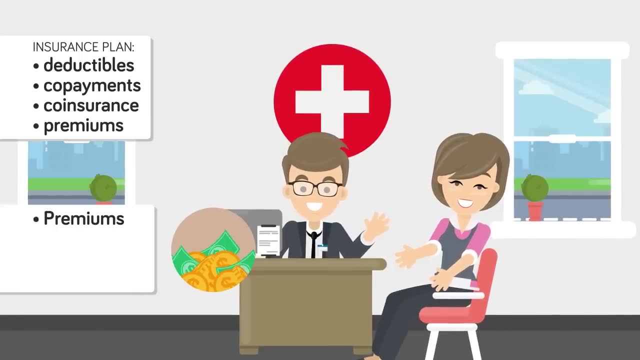 Deductibles, co-payments, coinsurance and premiums. The package you buy according to these things might save or break you. Premiums are what you pay, even if you don't make a claim. These can be very high. Co-insurance is a percentage of the cost you pay. A deductible is what you pay. 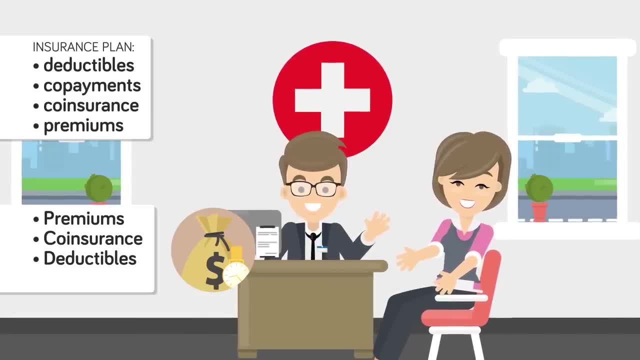 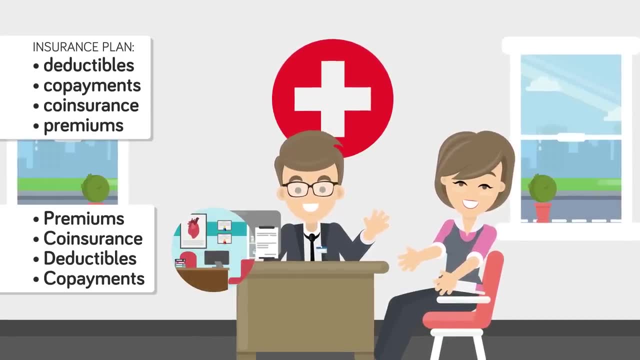 before insurance pays for anything, which can be as much as $10,000.. A co-payment is what you must pay for every visit to the hospital or clinic, and you'll pay that before the insurance company pays anything. So choosing the right plan is important, As one writer puts it. 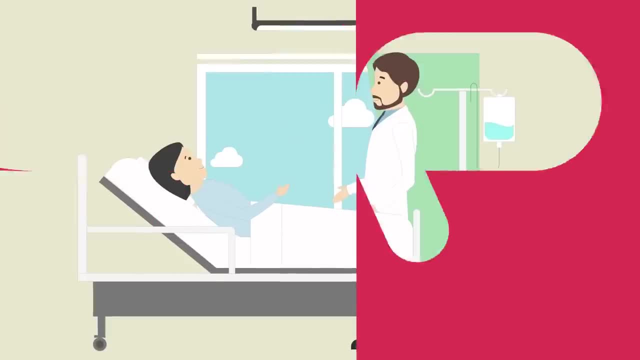 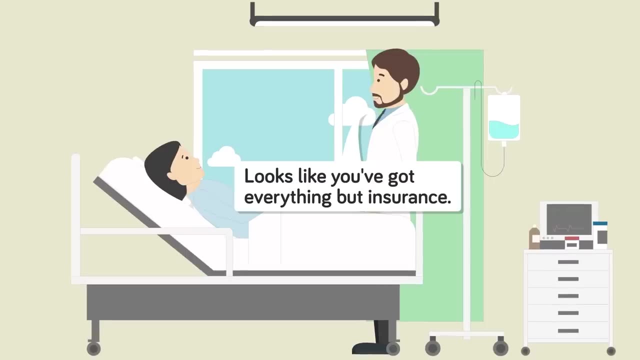 you've got to be an odds-maker on your own health. So what if you have no insurance? As we said, there are government-funded schemes for those in need, Also because of the Emergency Medical Treatment and Active Labor Act of 1986,. 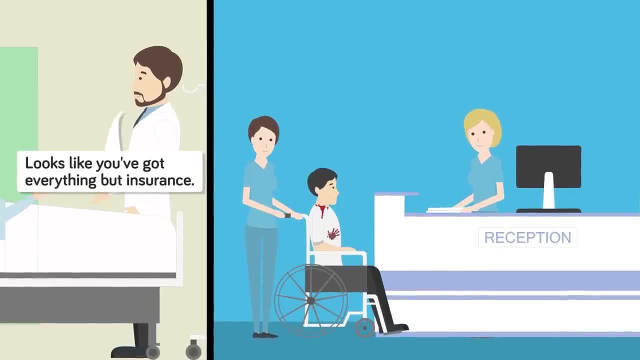 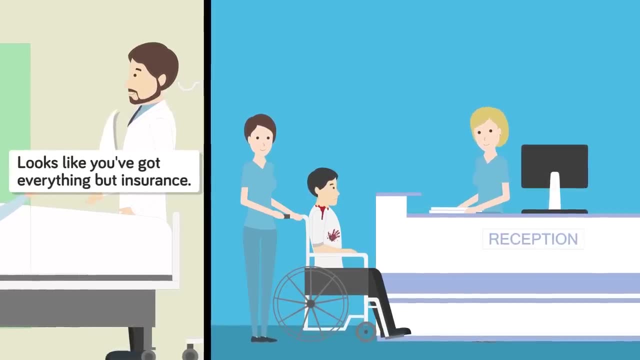 hospitals can't just turn you away if you're at the doctor with blood spurting from your neck. There's also the Hippocratic Oath, which means all doctors must try to treat you the best they can and do it ethically. But if you can't pay, there will be a bill, and in the US it will likely be. 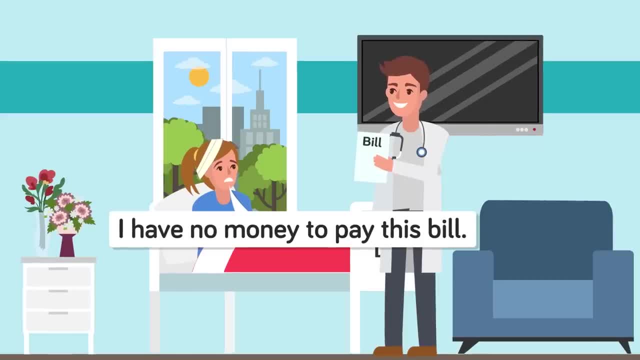 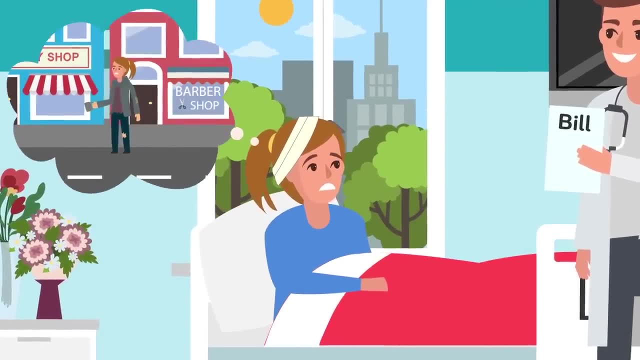 a large bill That could lead to debt collectors coming for you, your wages being garnished, part of the money taken out, your credit being ruined, having a tax refund withheld, someone wanting to take your house, or you could suffer bankruptcy. 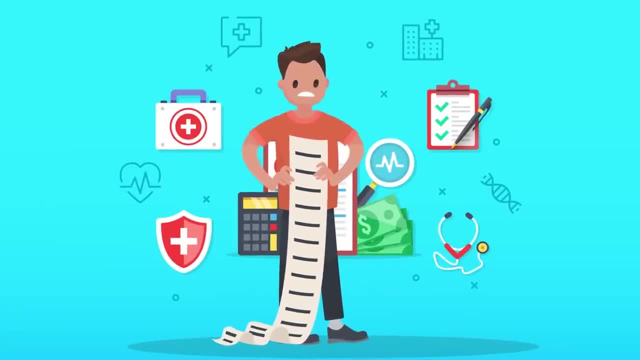 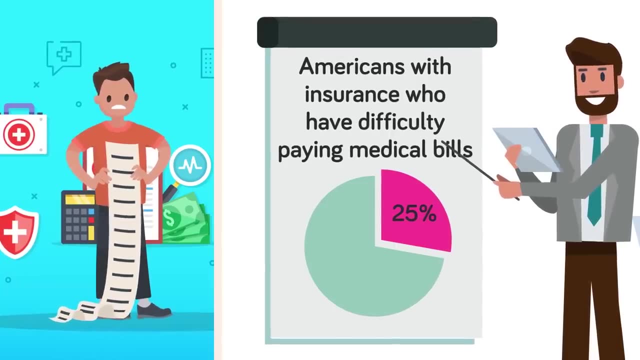 But surely those with decent insurance won't hit rock bottom? Not, according to the Kaiser Family Foundation That tells us more than 25% of US adults with insurance have difficulty paying their medical bills. You see, we are told that 63% of Americans who have had these medical bill woes 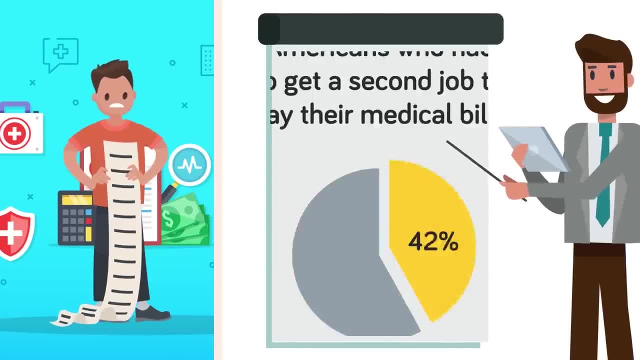 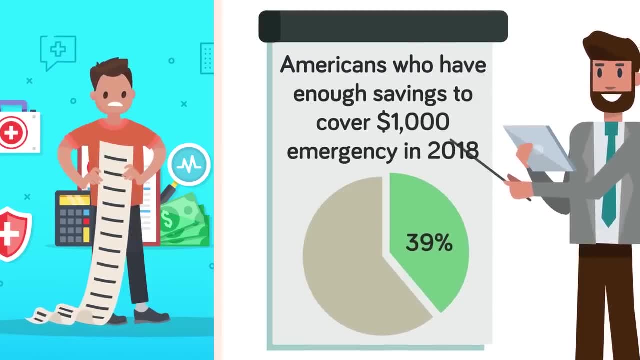 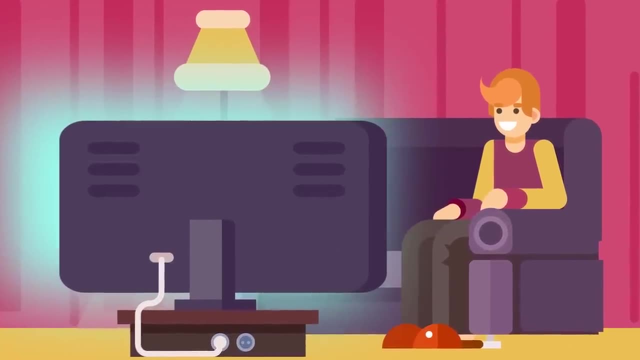 had to spend most or all of their savings on those bills. Another 42% had to get a second job. CNBC wrote in 2018,. Experts tell us Americans should downgrade their lifestyle in case they get sick, even if they have insurance, as going bankrupt could mean you might not get a loan again. 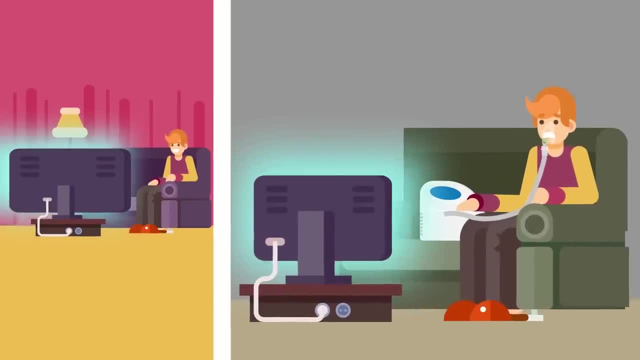 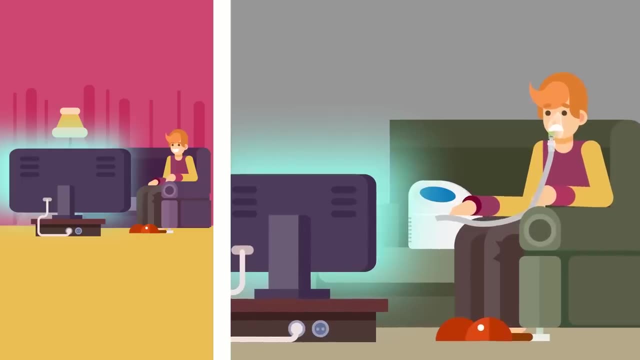 or be able to rent a house or even get a job. Sure, the poor and needy might get government help, but those that fall somewhere in the not-poor-but-far-from-being-comfortable category are often those who have to risk average insurance and the possibility of getting sick, ruining your 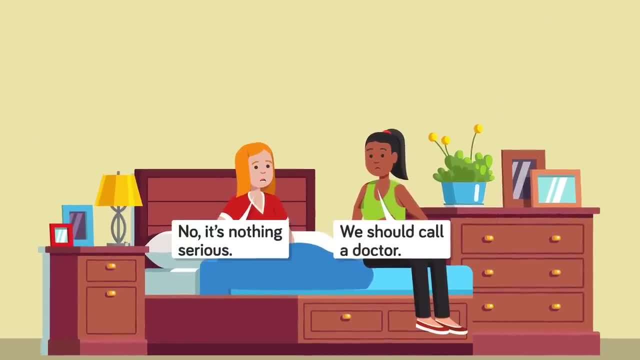 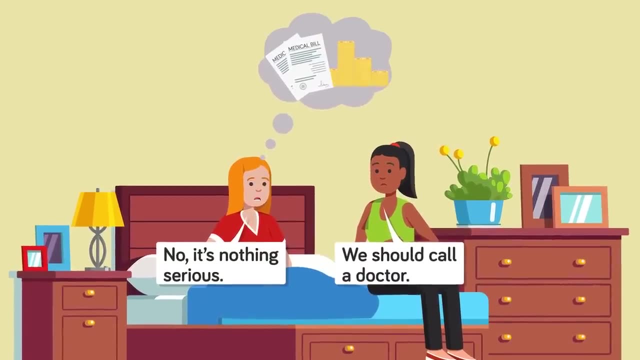 life. Another thing we are told is that 1 in 10 Americans delay getting treated because they are worried about the cost. That's what you might call a vicious cycle, because waiting can just make things worse. Some folks can't even afford the deductible. 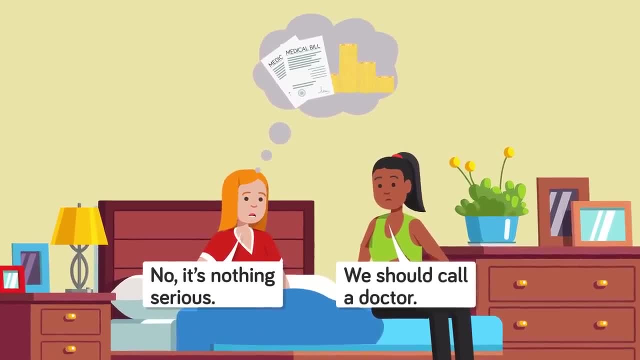 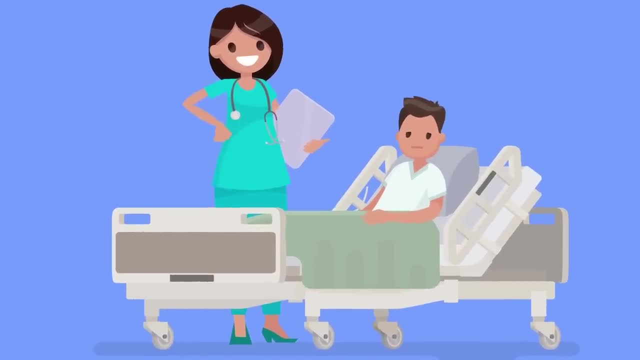 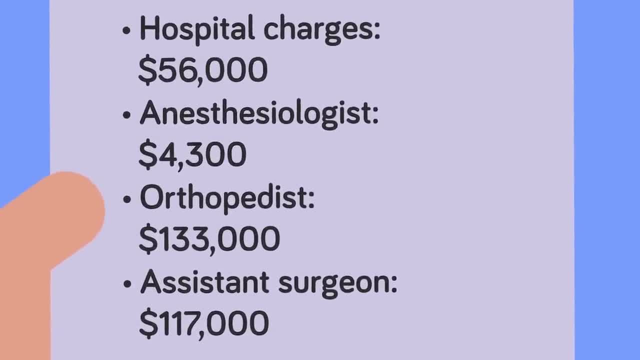 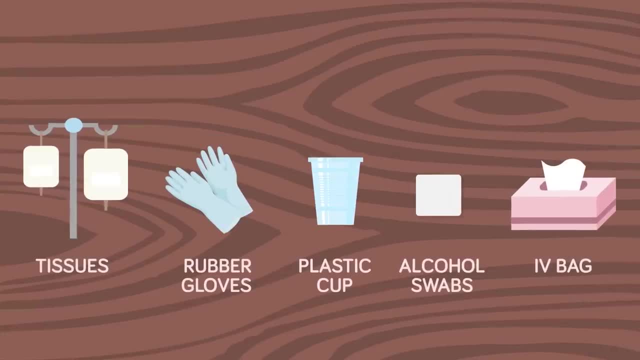 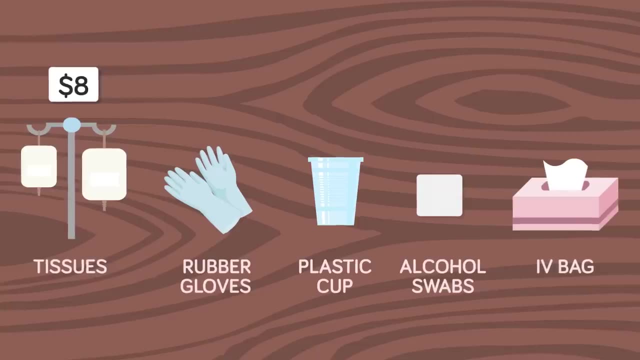 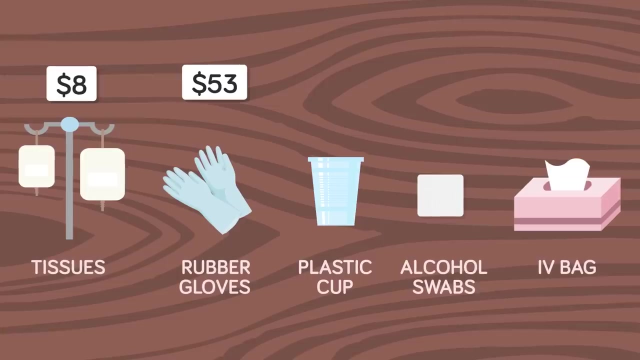 they want. We're told by Reader's Digest that some hospitals charge $8 for a mucus recovery system. They're usually called tissues. An investigation revealed one patient was charged $53 per pair of non-sterile rubber gloves. Sterile gloves were more Total cost for the stay just in gloves. 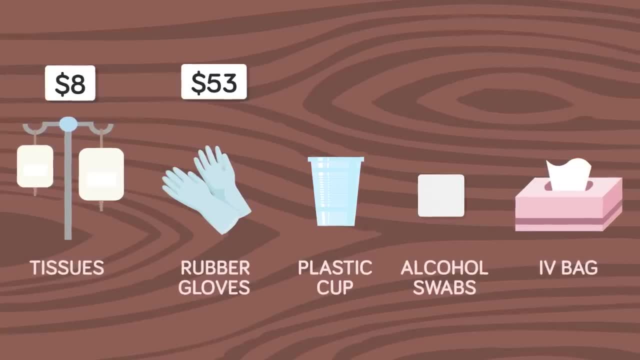 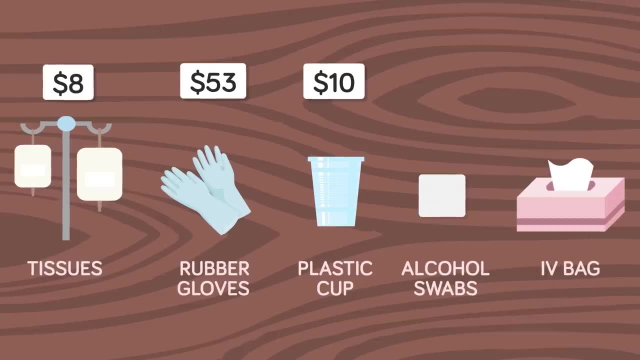 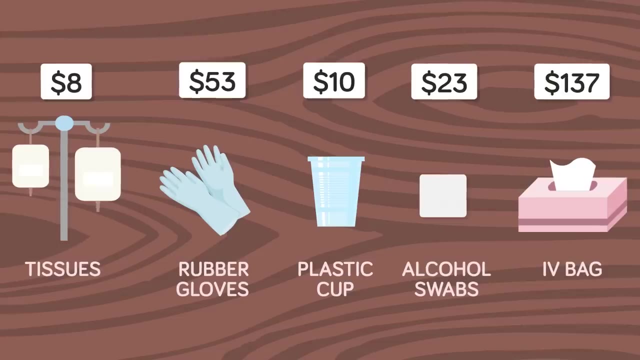 was $5,141.. That plastic cup they use to hand you your drugs- Ten bucks, with an average of $440 in cups for a patient's stay in the hospital. Alcohol swabs, of which you may need many- $23 a time. One person was charged $137 for an IV bag. The cost of that bag: $1.. This is mostly due. 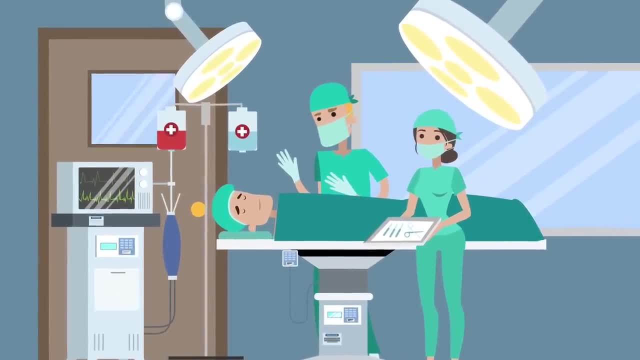 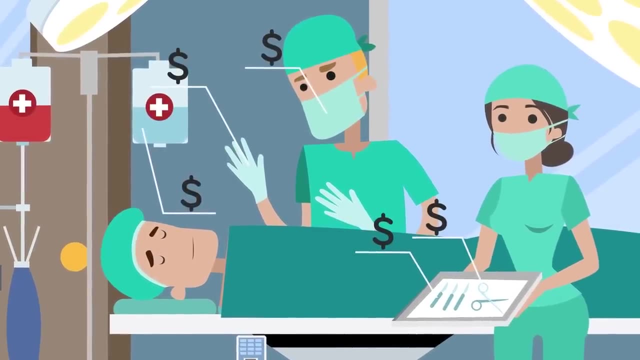 to something called the charge master, which allows hospitals to charge out-of-this-world prices. These codex of costs are hospital services, hospital insurance, hospital insurance, hospital specific, meaning each hospital makes up its own prices. Some critics have called such costs. 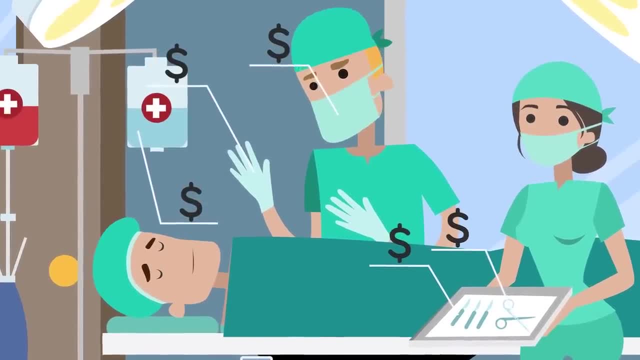 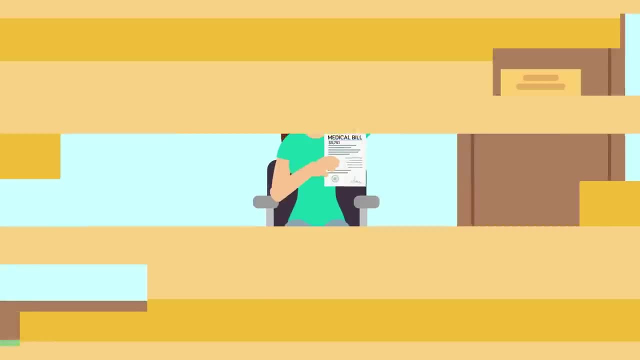 fiction and are critical of the lack of transparency hospitals provide about this hidden menu. The loser, of course, is the consumer, whose life may depend on that five-star menu. Vox reports that one woman who hit her head and went to the ER left with only an ice pack and